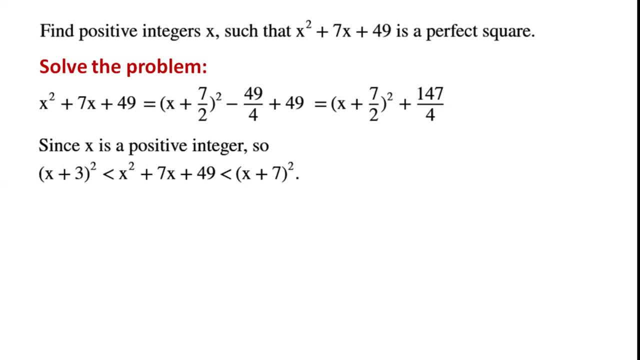 x squared plus 7x plus 49,, which must be less than x plus 7. all squared, x plus 3, all squared, can be written as x squared plus 6x plus 9, which is less than x squared plus 7x plus 49, as 6x is less than 7x and 9 is less than 49.. 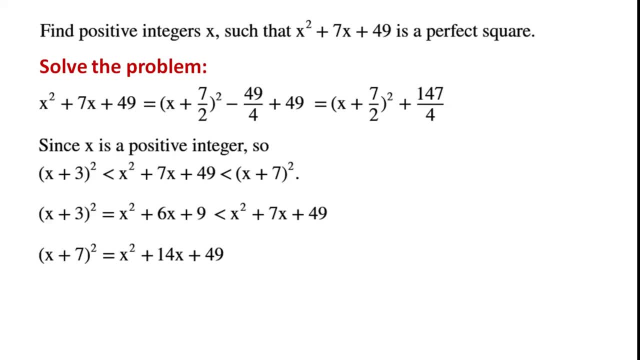 x plus 7 all squared equals x squared plus 14x, x plus 7x plus 49,, which is greater than x squared plus 7x plus 49,. as 14x is greater than 7x plus, the perfect square can only be x plus 4 all squared. x plus 7x plus 49,, which is greater than x squared plus 7x plus 49,, as 14x is greater than x squared plus 7x plus 49,, which is greater than x squared plus 7x plus 49.. 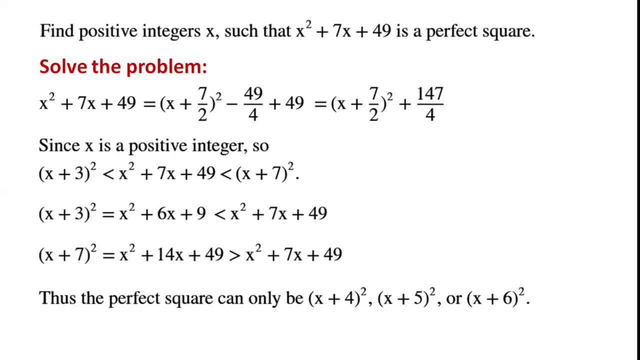 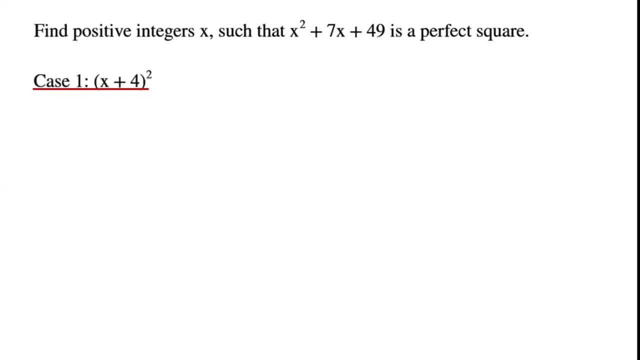 x plus 5 all squared or x plus 6 all squared, Case 1. If the perfect square is x plus 4 all squared, then x squared plus 7x plus 49 equals x plus 4 all squared, which can be written as: x squared plus 8x plus 16 plus x equals 49, minus 16 equals 33..